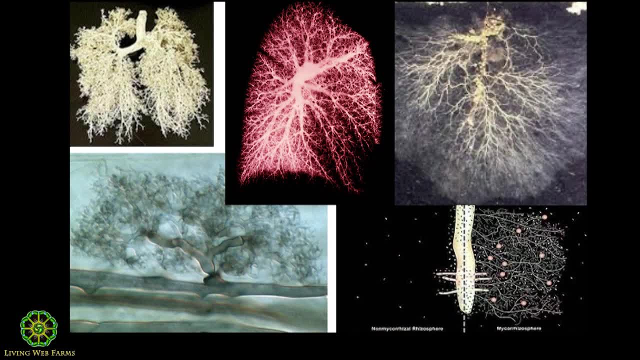 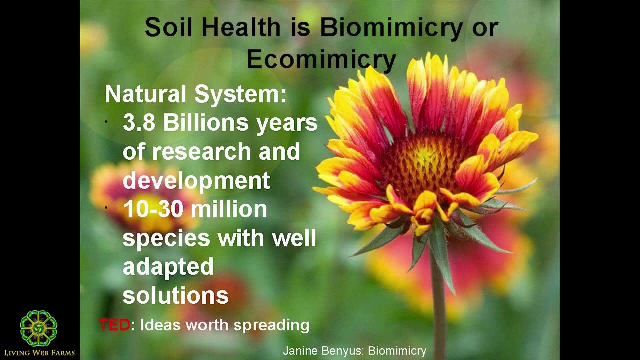 know I want you to understand cycles, patterns, understand nature's connected. Okay, here's what we're going to follow. If I use one word for soil health, everybody write this down. you should see her video. Jeanine Benyias, Write that down on TED. It is two 20 minute. 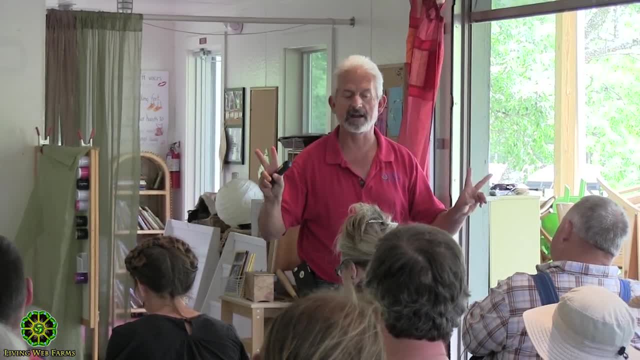 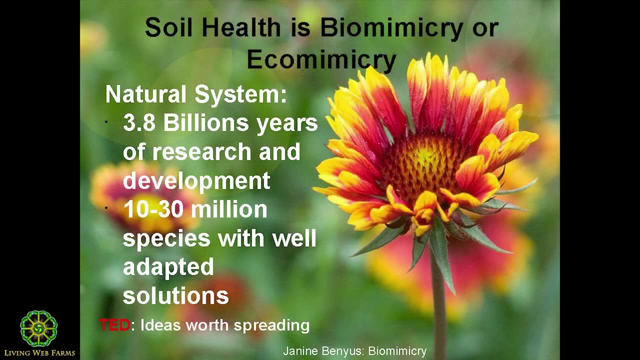 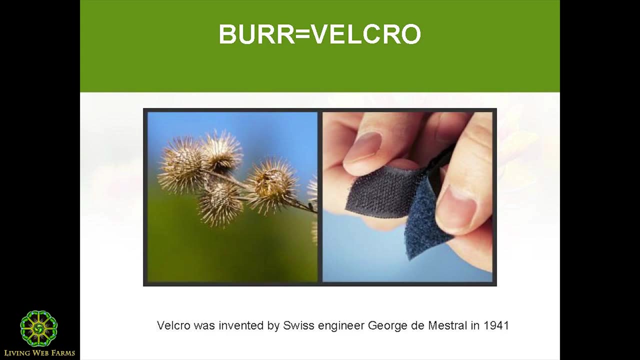 videos of awesomeness. She is incredible. She's got whole talks that nature uses 3.8 billion years of research in 10 to 30 million species for well adopted solutions. Sorry, Do you know that Velcro was designed by the burr? 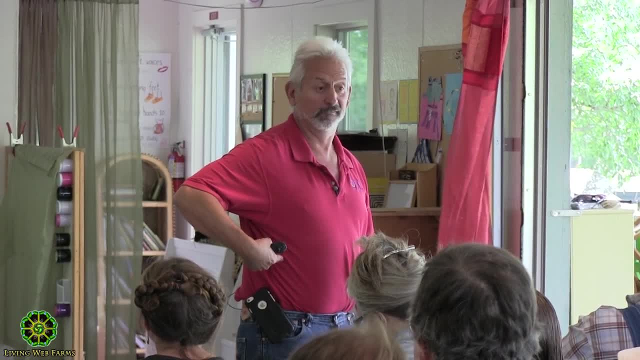 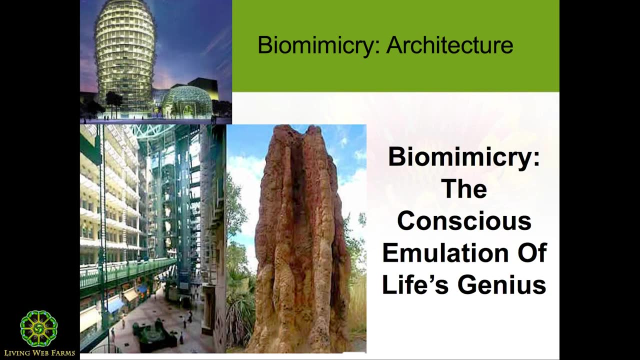 The engineer sat on this dog's fur and said: hey, what do I make? Velcro Millionaire? She argues, let's learn some more here. Do you know? this is in Africa. They're using the termite mounds to mimic their air conditioning system. 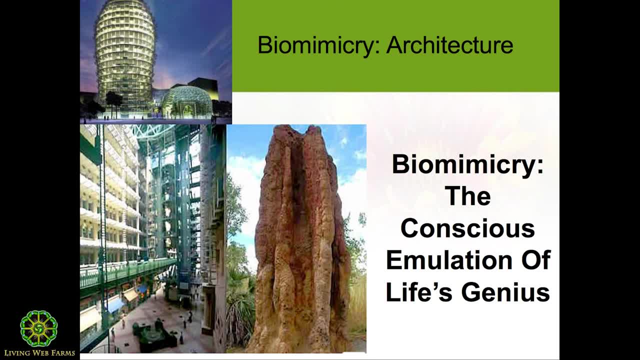 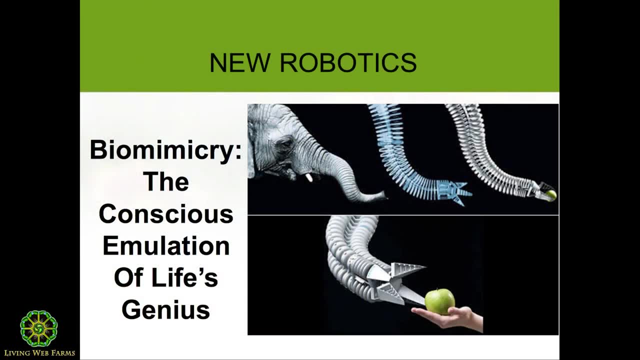 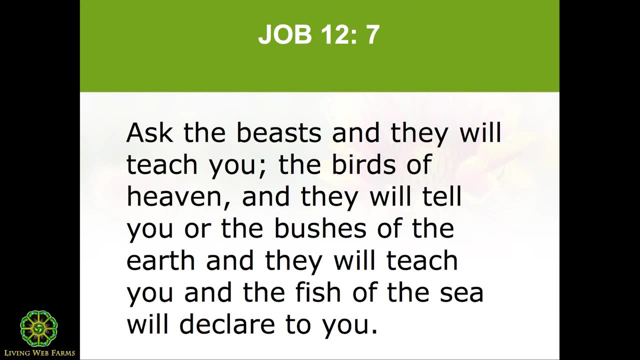 and they're putting in buildings, reducing their energy input by 90%. Biomimicry, Biomimicry, new robotics, elephant trunk Biomimicry has been around for a long time. folks, Ancient scriptures, say: watch the beasts, look at the animals. 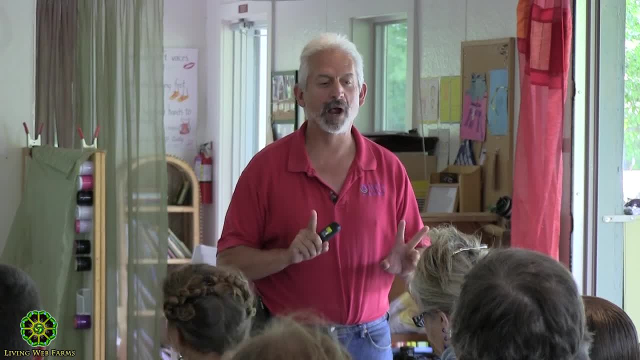 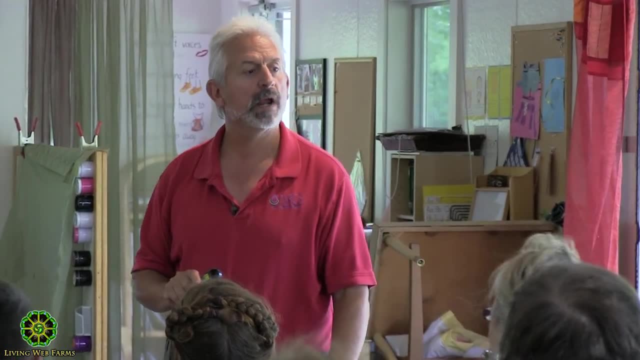 Do you know how? I never knew about biomimicry. My education got in the way. Eight years of college got in the way. What did Einstein say? Never let your education get in the way of your learning. Neen, Okay, here's how we're going to mimic today. 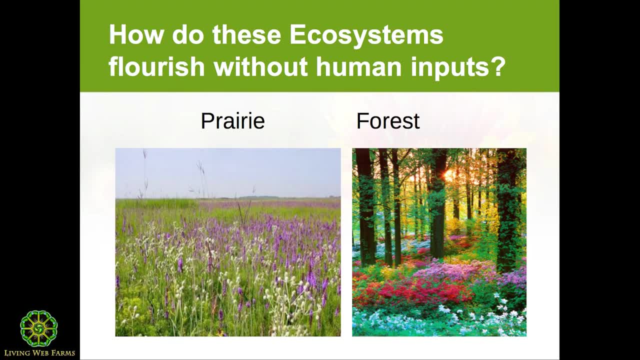 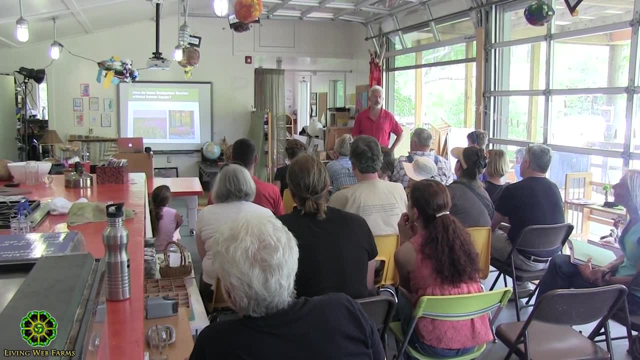 Prairie and forests. What do we see here that we want to mimic? What are the principles we talked about? Come on, audience. What does a prairie and forest have in common? right there? Diversity. What else? Come on, Feed me. 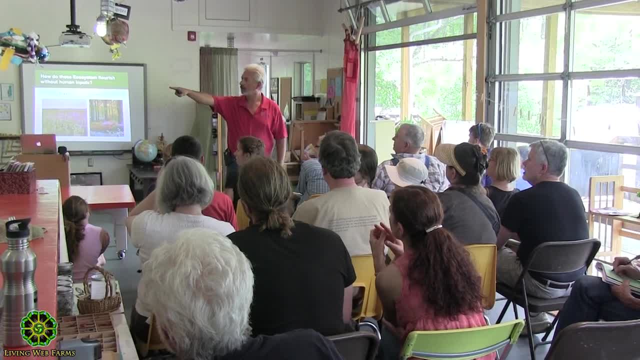 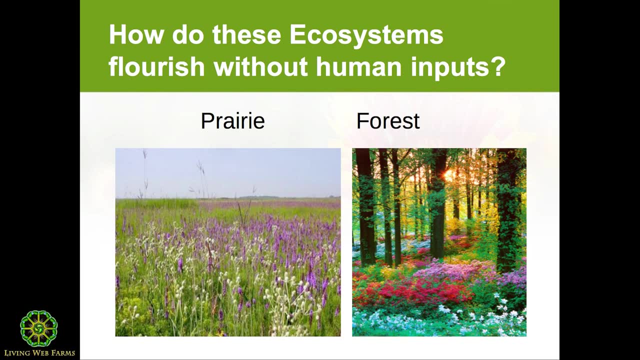 Give me goosebumps here. Work with me. They got synergy. What else do you see out there in those pictures? They're covered 24-7.. Do you see the co-op fertilizing it? What else is going on? Diversity. 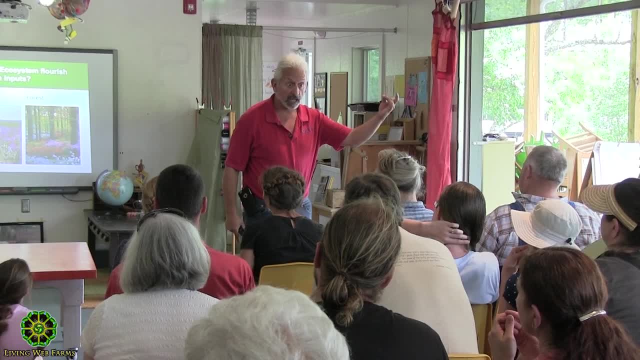 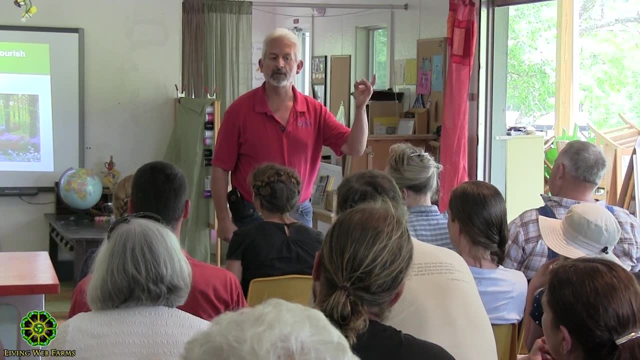 It's covered. What else Is it covered 24-7?? Yes, Yes, Yes, It's diverse, it's covered. we're missing some other ones. Come on, They both have animals in the system, right? So guess what we did in our agriculture systems. 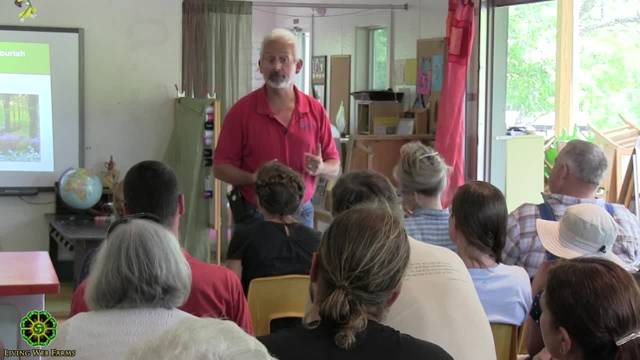 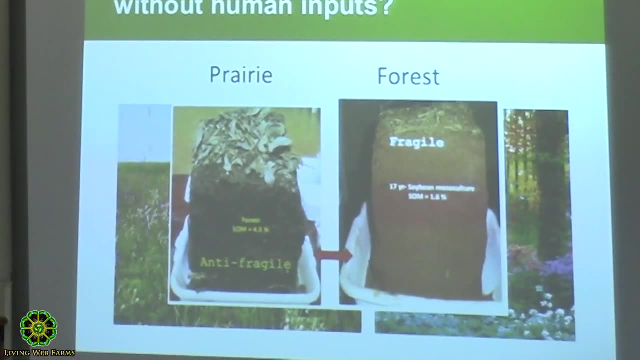 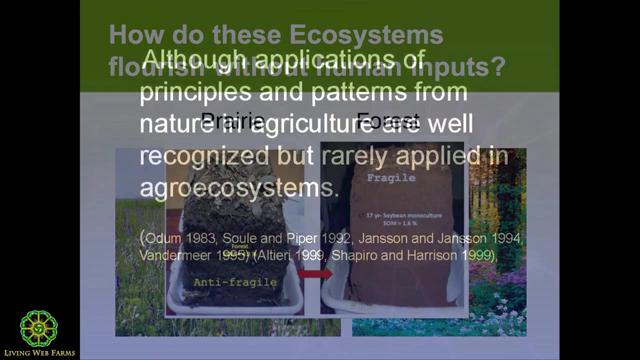 They're not covered, they're not diverse and they have no animals in the system. They're in feed lots, Okay. So look at the soils. differences Forest, the way we farm same two soils soils. Now some people say, well, Ray, you're making all this up. Really, Pat, look at this. 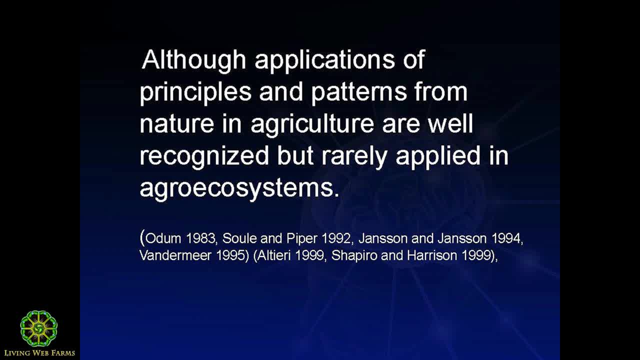 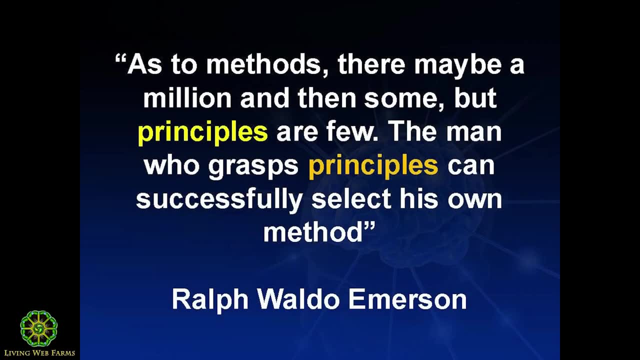 Dr Odom, Piper Jensen, Dendemir Terry, all these guys says nature has principles that should be applied in our agroecosystems and they should have been there for years. We've known this. We've known this. Okay, The principles are constant, The methods are different. If I 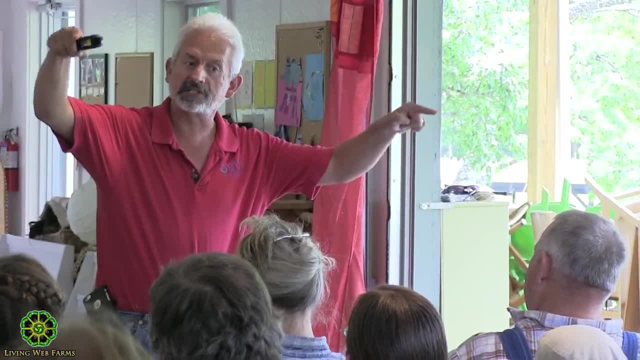 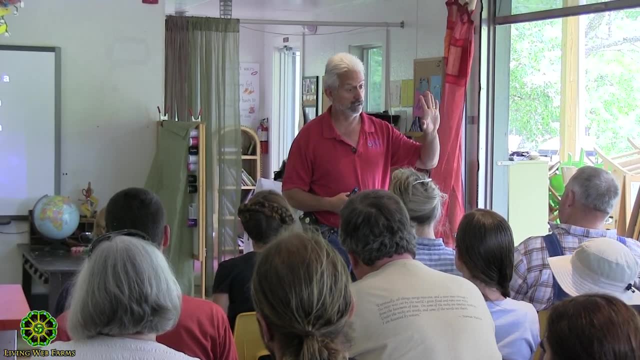 send you to Kansas. you're still going to apply the same principles, but the methods are going to be different. Kansas only gets western. Kansas gets 15, 16 inches of rain. Should it still be covered, You better believe it. I should be more judicious with the principles, In fact. 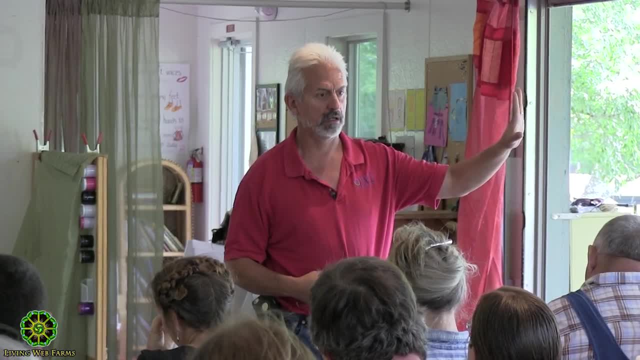 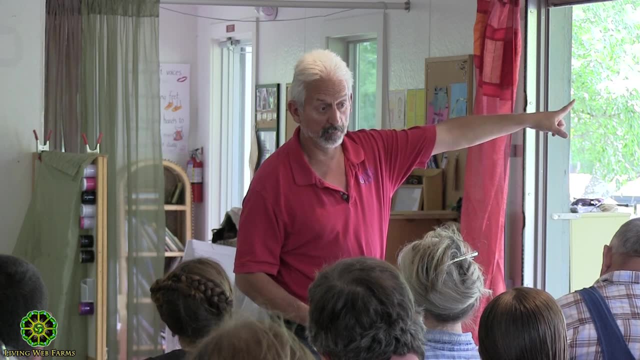 I mimic the prairie over there. You should probably not be farming there. It should be more grazing systems. Okay, Your template's right there. Your template's that forest I'm going to show you as we walk in the field today. 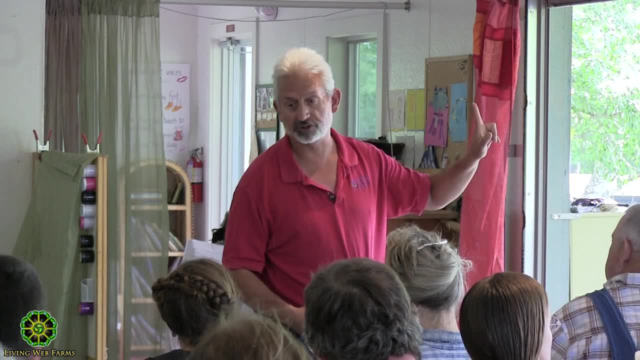 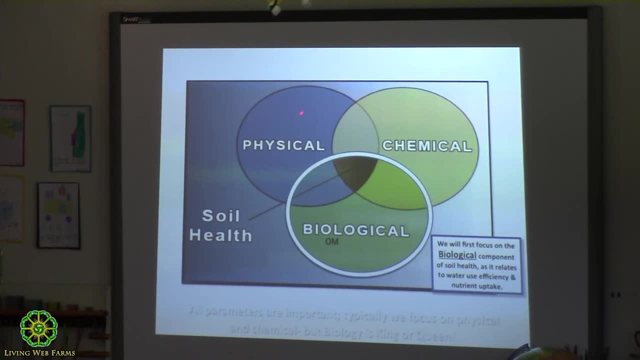 how the forest soil looks and comparing to some of your soils. Okay, Now we've been taught this. everything has the same parameters. Well, I'm going to hear to tell you, folks, these are not equally important. This is what it is. Biology builds the physical. and it helps regulate the chemistry Who builds organic matter? Biology does So. you can hold more cations, You have more regulation. That's why your soils are highly buffered. That's why they say highly buffered organic matter. So there's biology. Now I'm going to ask: 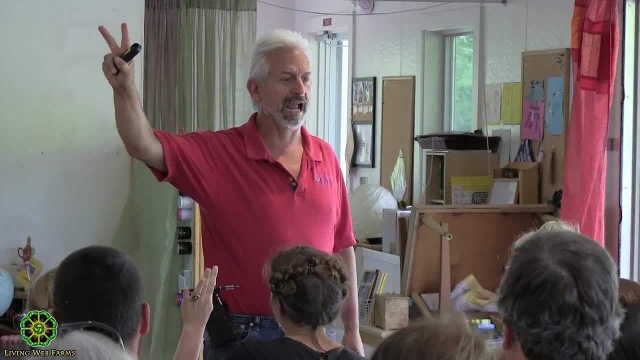 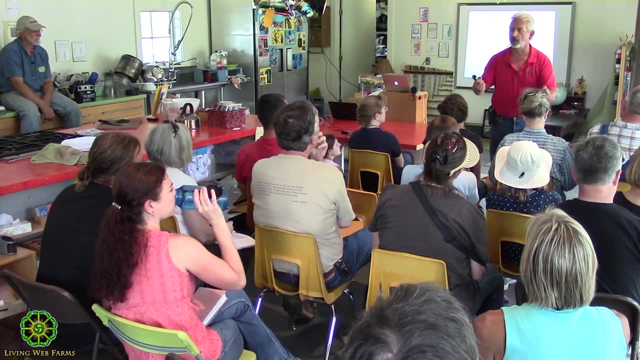 everyone. how many of you guys farm in here? Raise your hand. Okay, How many of you use this tool religiously? And you're walking through every one of your fields and smelling your soil, counting earthworms, looking for aggregation. Religiously, raise your hand. That's what I thought. 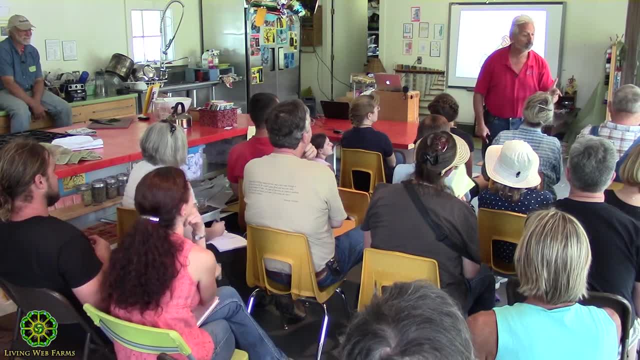 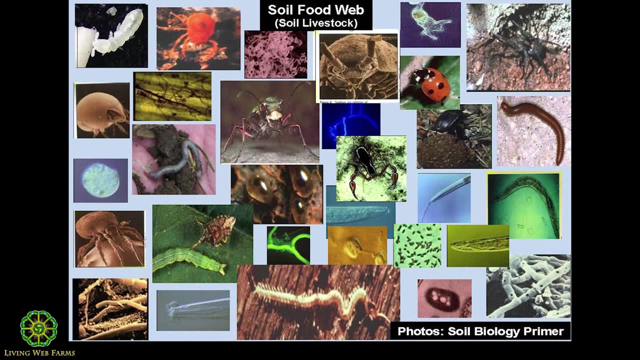 You know what we do now. I don't walk out until we pull a shovel, didn't we, Dave? What's the first thing we did on the farm? We dug a shovel right, Pat. Okay, this is what I want to see, Because why? There it is. This is what you're dealing with. It's a 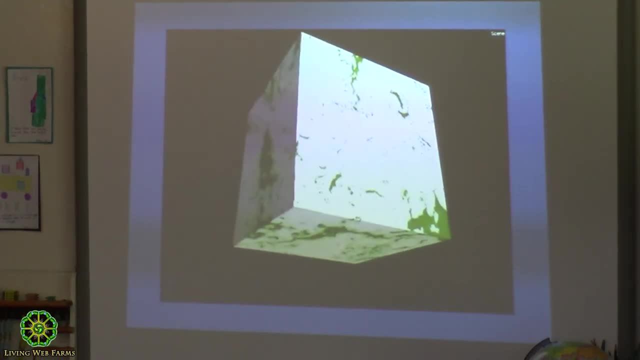 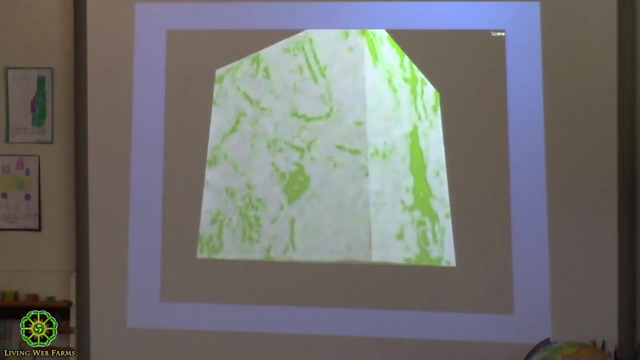 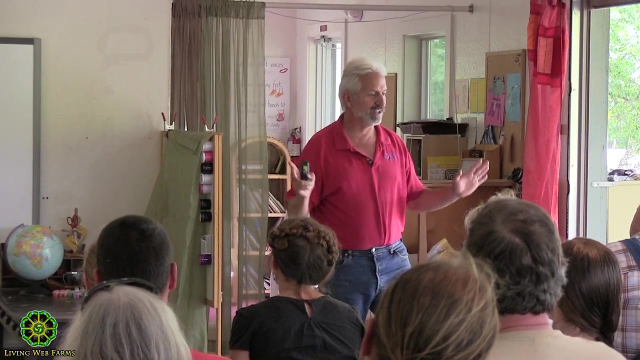 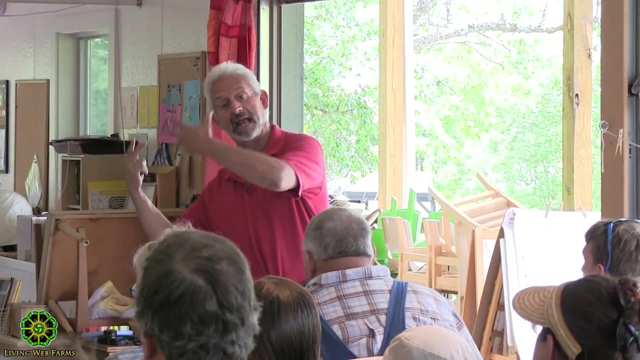 aquatic ecosystem. It runs on water and carbon. Okay, look how elegant That cottage cheese. those aggregations are fused together to make a subterranean universe where all these organisms live. What do you think, Andy? one tillage pass does Destroy them. Yeah, let's mess up the house and then we'll build compost and bring it. 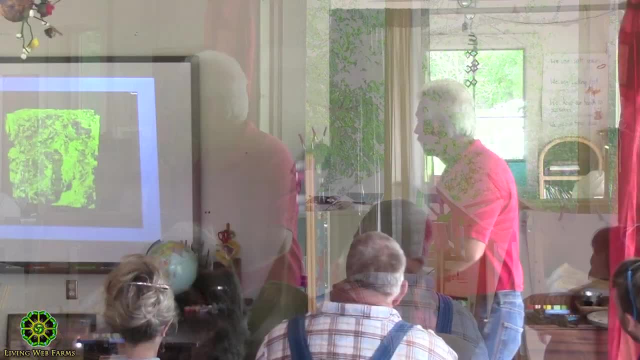 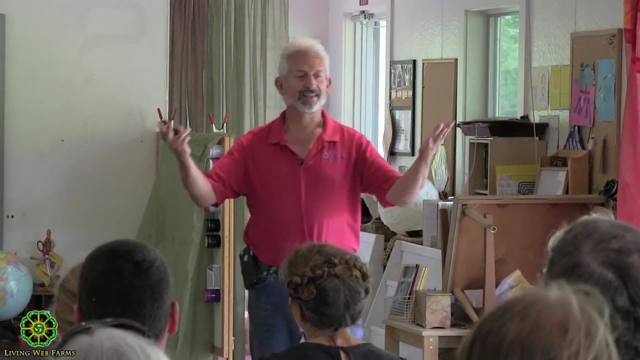 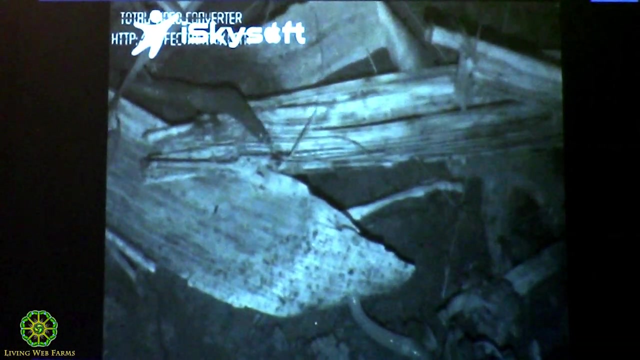 back in and use ancient sunlight. We can use covers and reduce that. Now, how about this baby? Now, this is emotional, Right here. Look at that. I just wanted to touch your heartstrings right there. Look at that. This one. 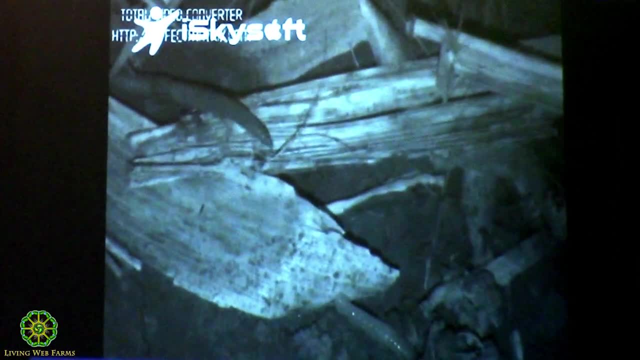 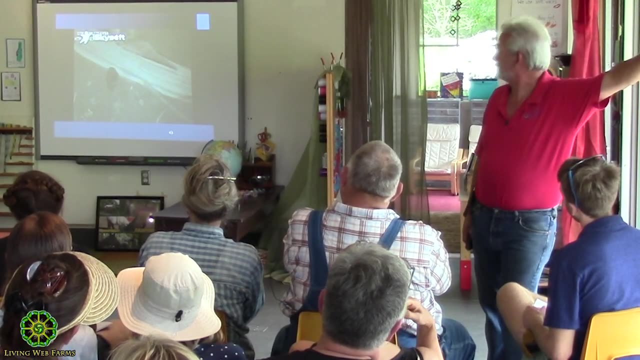 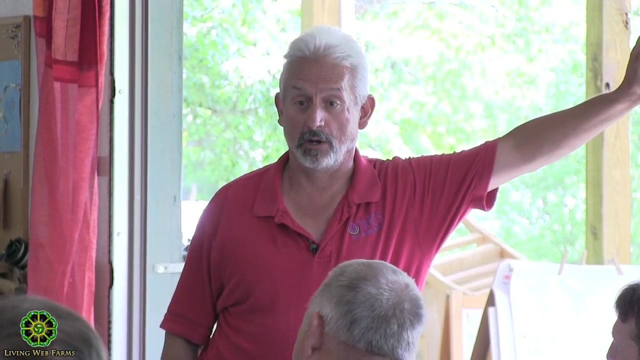 was taken in a no-till field in Quebec, Canada. A special camera at night, Look it. I never thought earthworms would do that. Whoa, Isn't that cool. Do you know? they can take a whole forest floor down. 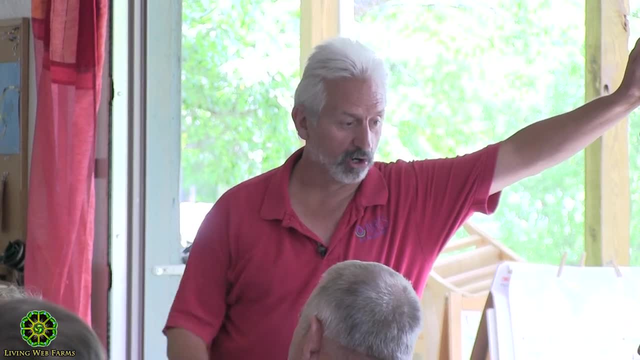 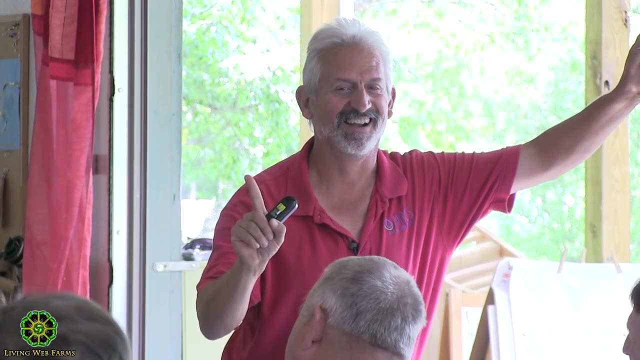 in a whole summer. They want food. So this is why David Brandt does not go at his field by himself at night. He'll disappear. Where's David? Oh, they took him. All you hear is earthworms going. They got him, man. 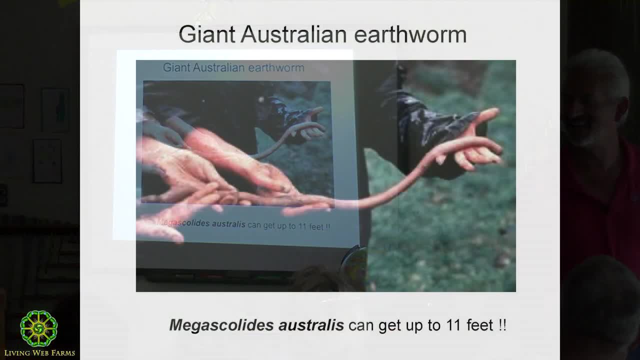 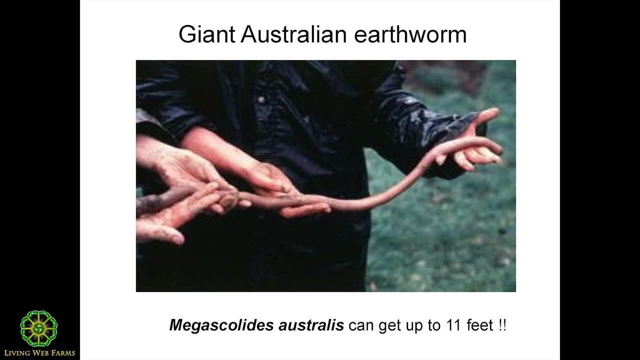 Poor, poor David's gone. How about that earthworm? I said, Mark, you go check the field. No, you go check it. Ah, that's Australia. I'm not going out there. uh-uh. Now, why do I care? 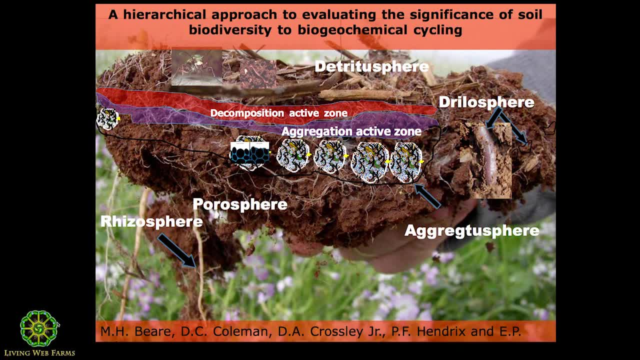 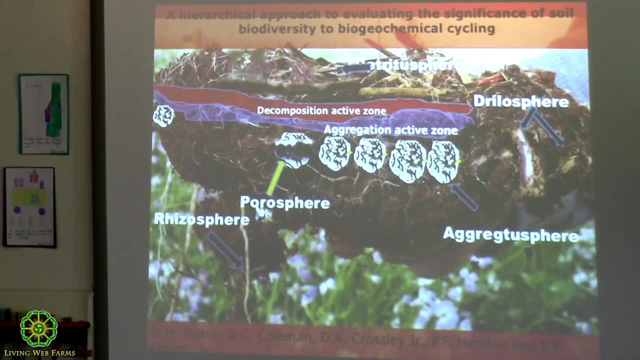 Okay, now when we go out in the field today, this is one of all the spheres I wanna see present. We're gonna see in the gratisphere, drillosphere is the earthworm. We're gonna see the detritus sphere. 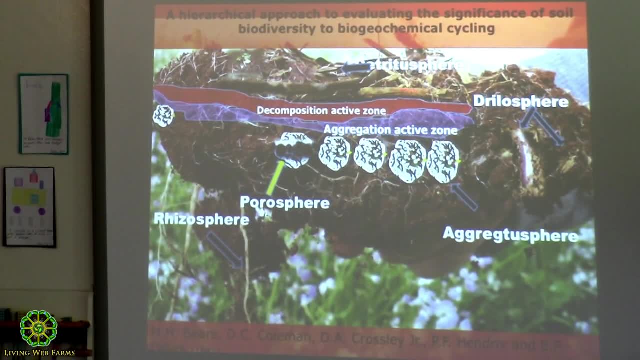 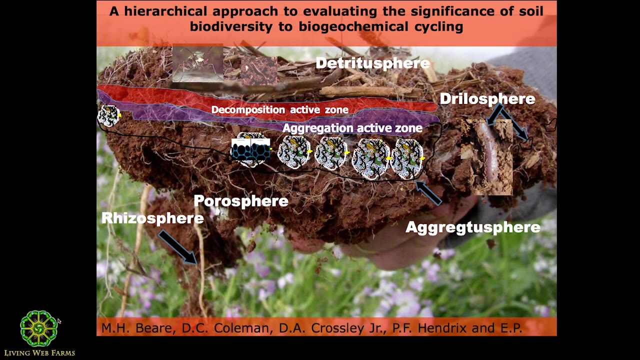 That's the residue. Agratisphere is the cottage cheese. This is the residue sphere Inside the cottage cheese are porous and rhizosphere. We're gonna see where we wanna see all this present This look, oh research. Baer, Kullman, Grosley, Hendricks love this. 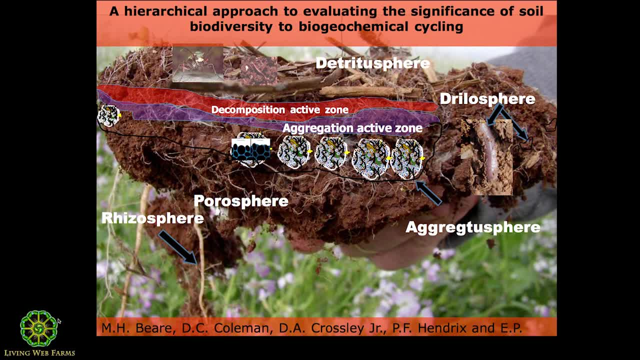 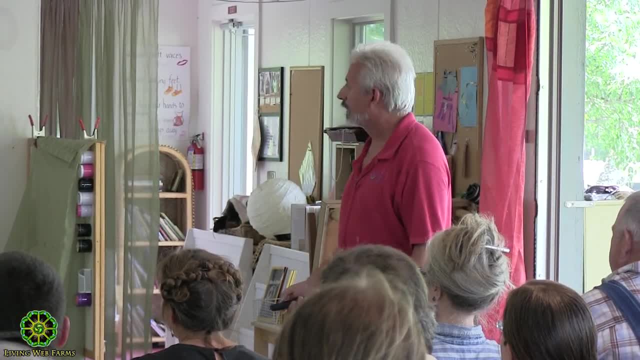 Paper: hierarchical approach to evaluating the significance of soil biodiversity to biogeochemical cycling. Say that quickly. How old was that? It was published in? it was done in 1995. 1995. 1995. 1995.. 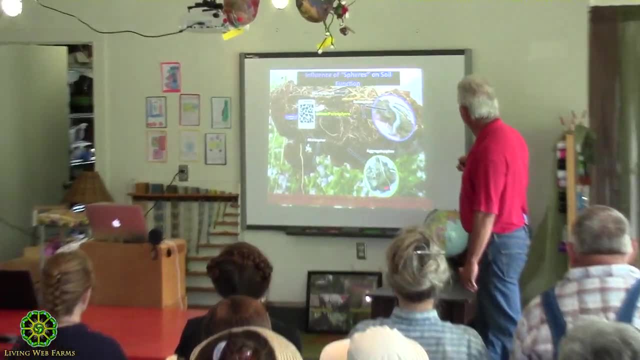 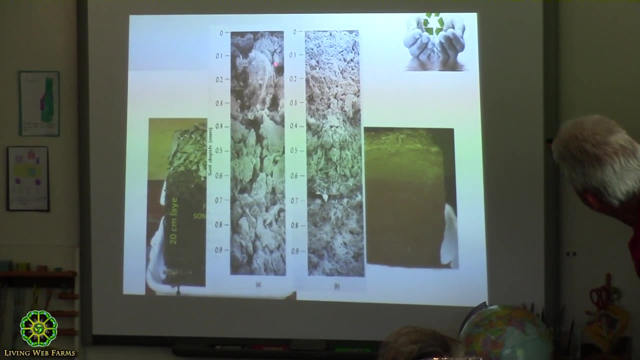 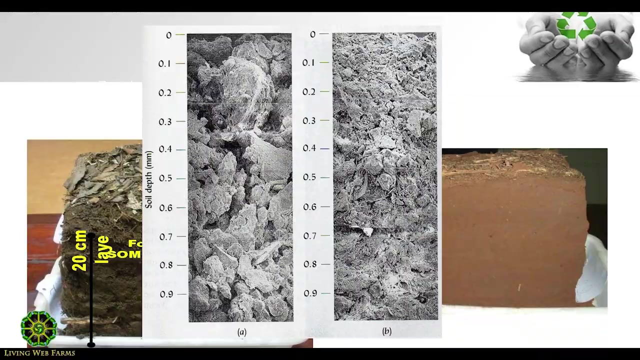 1995.. Great paper. I definitely recommend it. So we're gonna see this Now. electron microscope: no-till field up to nine millimeters. Look at the top of the pores. Look at a conventional field. Remember why I was telling you the water don't infiltrate. 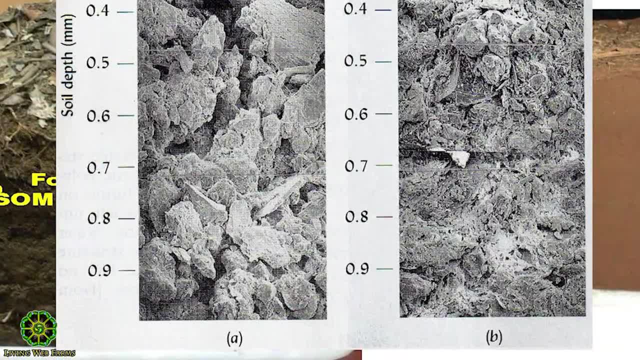 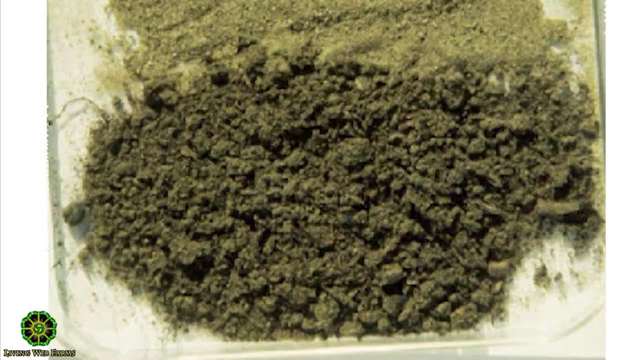 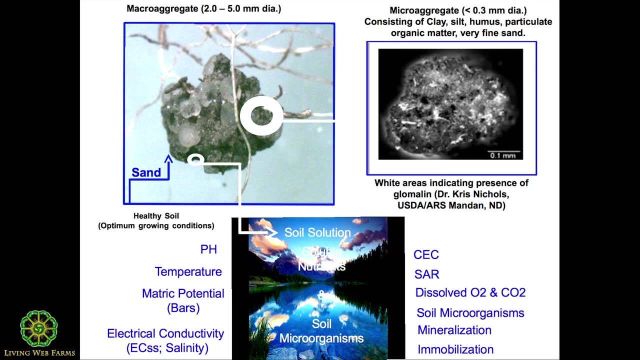 Look at here: Electron microscope. Okay, Now here's what I wanna see. Look at the cottage cheese tilled no-till. This is what we're gonna see today when we go in the field. Look at this: How many have sandy soils? 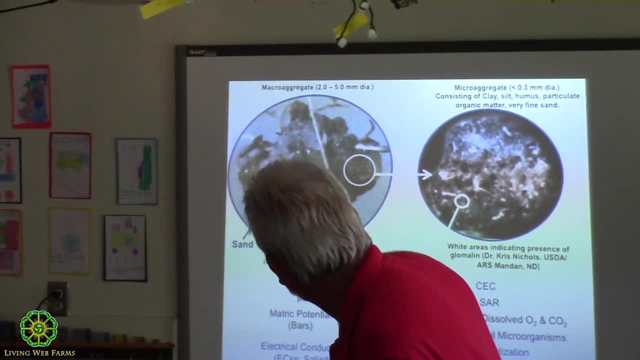 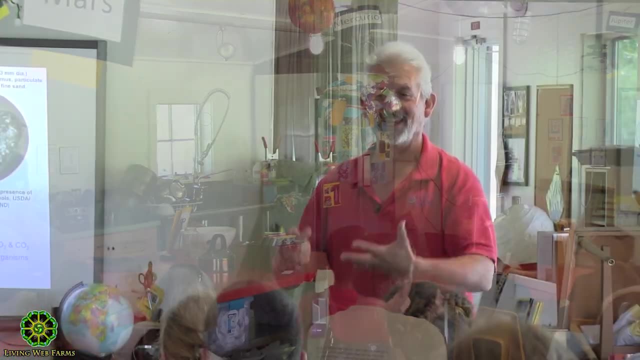 Look at here, Pat, Those are sand grains, Became dark-coated. Now, Pat, how did they come coated like that? Microbiology, Biology, The biology, the metabolic: they coat those particles. Look how dark it gets coated. 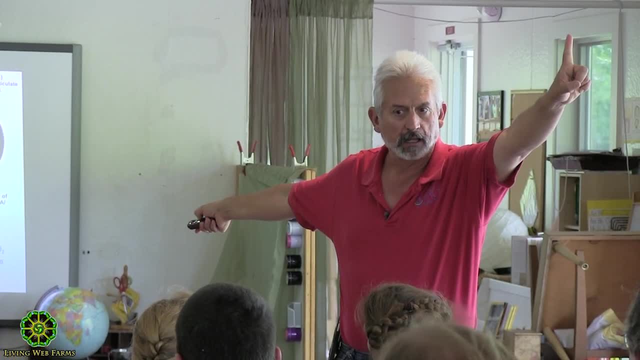 Now I have cation exchange capacity, Now I can hold on to nutrients. That's sand. I've seen no-till sand dark getting coated with those particles. Now, okay, compaction. How do we fix compaction? What is your name back there? 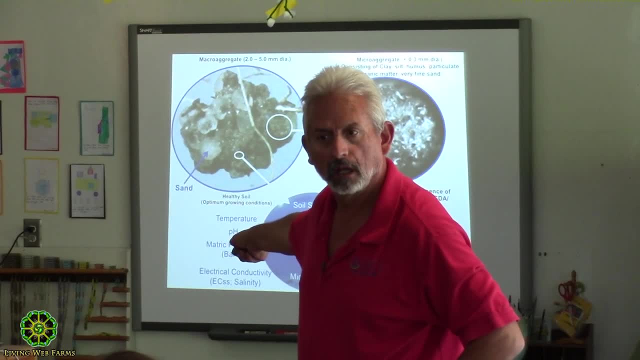 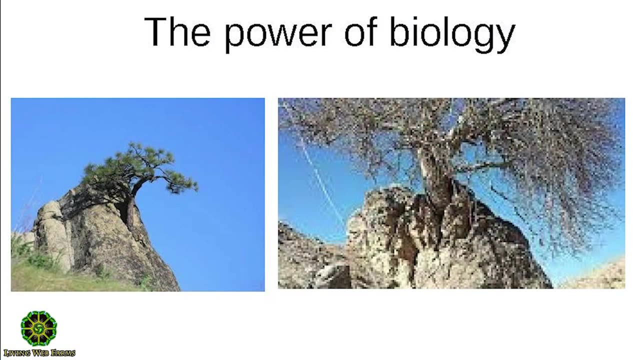 Tom, Tell me, Tom, How do we fix compaction usually? What do we do? What's a typical farmer thing we do for compaction: Horsepower, right, baby, Horsepower, Horsepower, Horsepower, Horsepower. 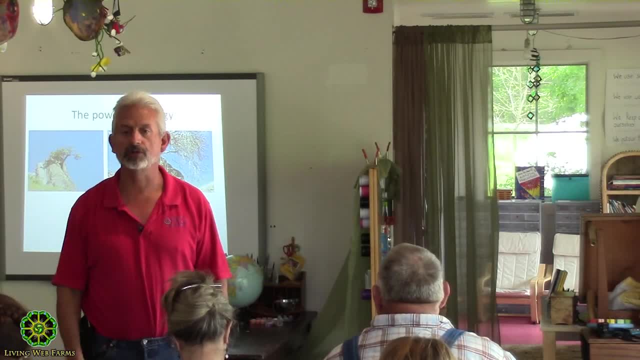 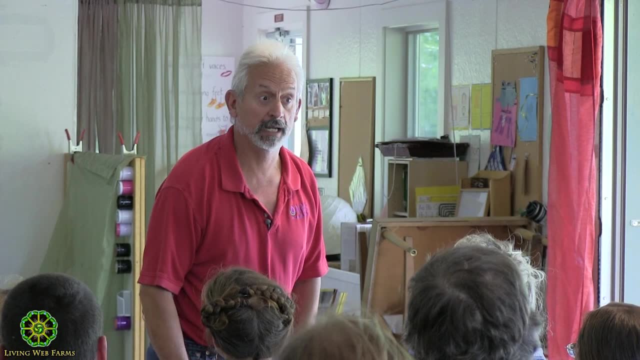 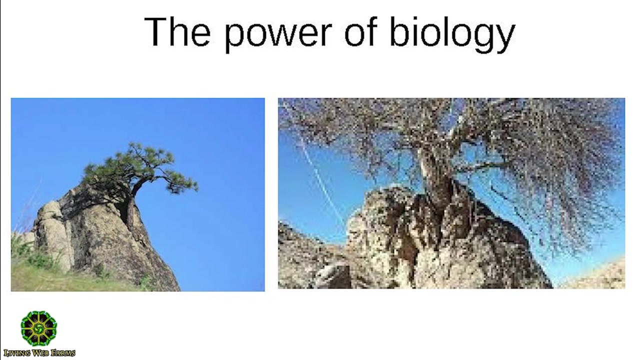 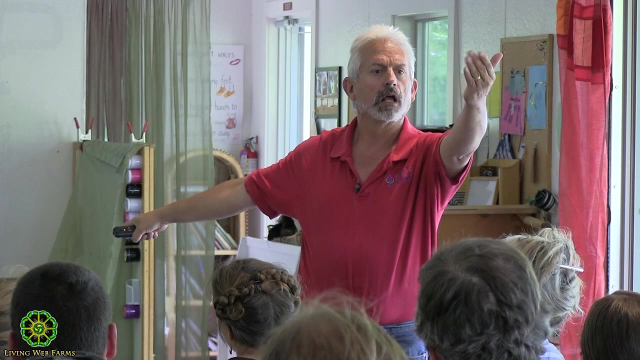 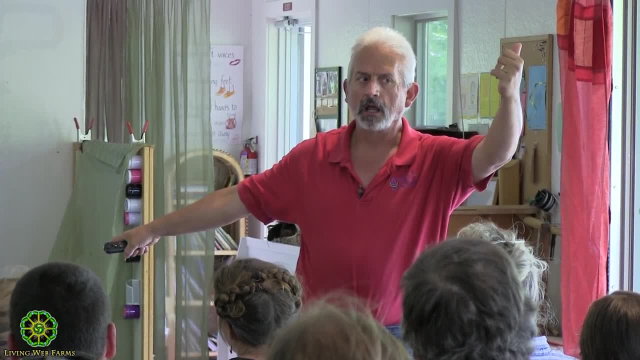 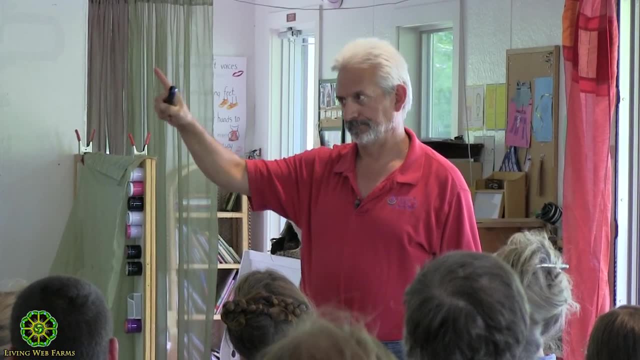 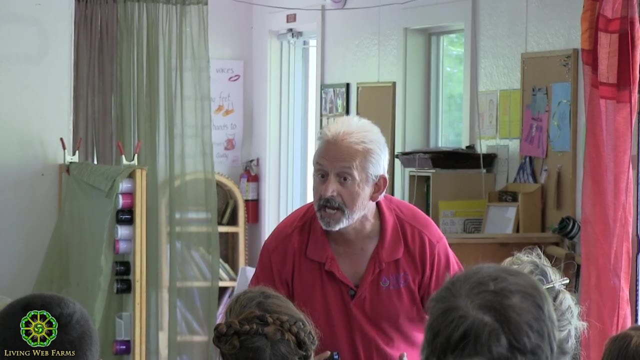 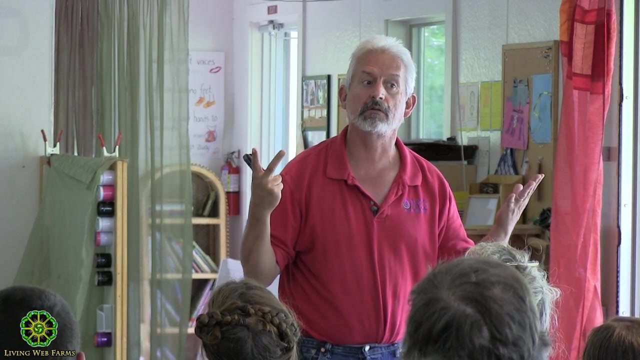 more. what's going on? that's rock. that is rock, guys. okay. so as they're respiring, they come in contact with water. they release carbonic water and co2s, carbonic acids, exoenzymes, the mycorrhizae and the bacteria. you can break those inner. 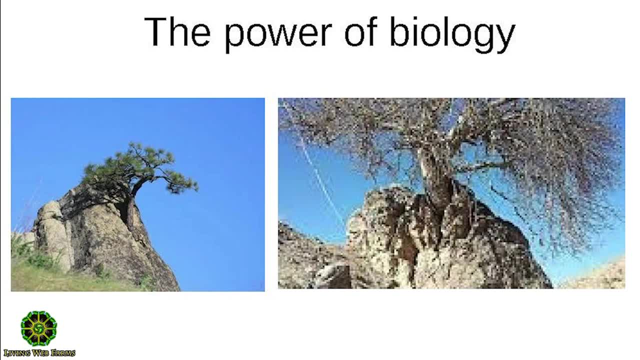 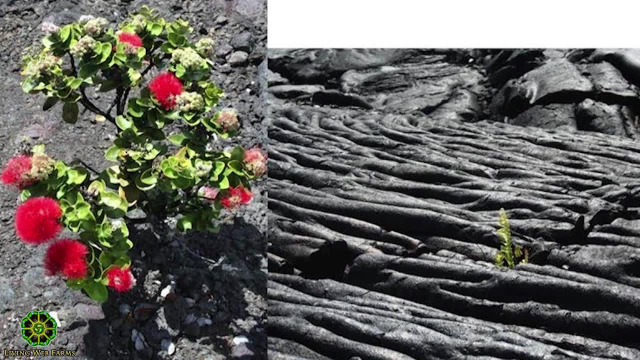 inorganic substances and get make their living off it. biology: oh, I took this in Hawaii five months ago. that is solid lava. how is that growing there? little bacteria, the spores, land seed, lands in the crack water gets in their primary succession. it takes a foothold. these. 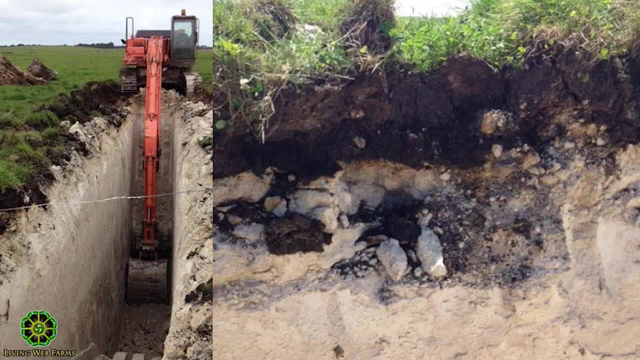 plants release these powerful acids. how would you like to farm this, Dave? you know what that is Australia. you think you have it tough. look what they have. I have a question for you, audience. how come this is not the same color all the way through? that's calcium deposits of an old ocean bottom. 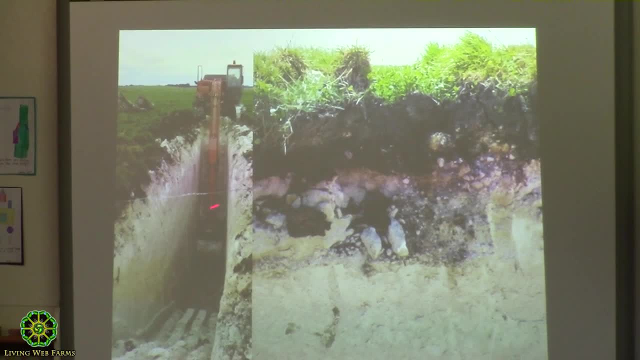 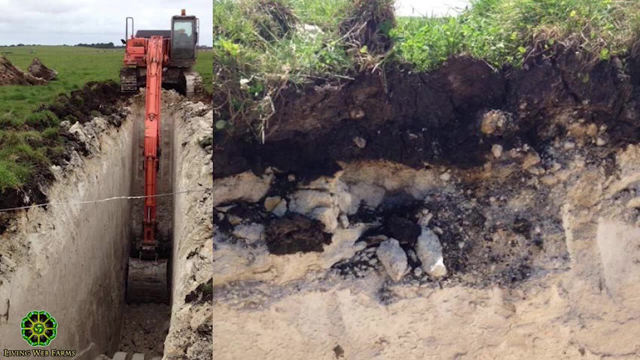 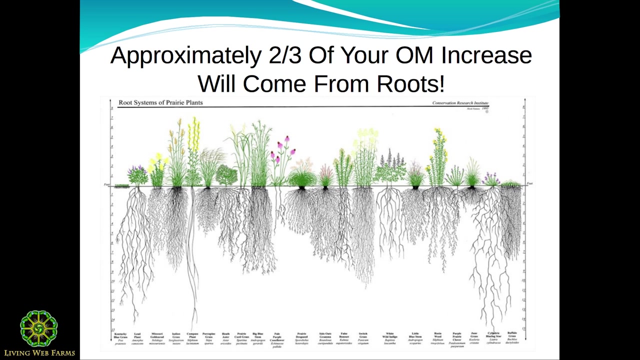 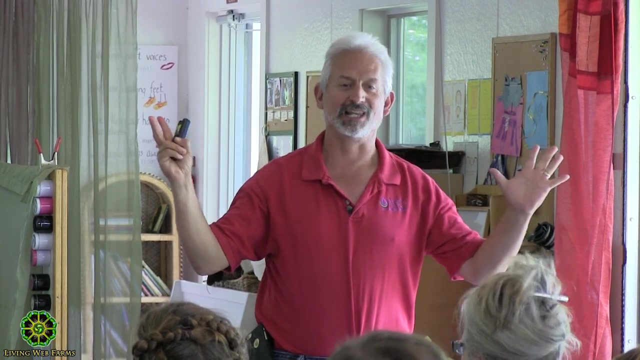 yeah, look at the biology taking the foothold. I want you to walk away. how powerful it is. do not underestimate the power of the biology. okay, our mixes are gonna look like this. why do we want our cover crop mixes to look like the prairie? different depths to have different canopies. this is what we're bringing, ecological. 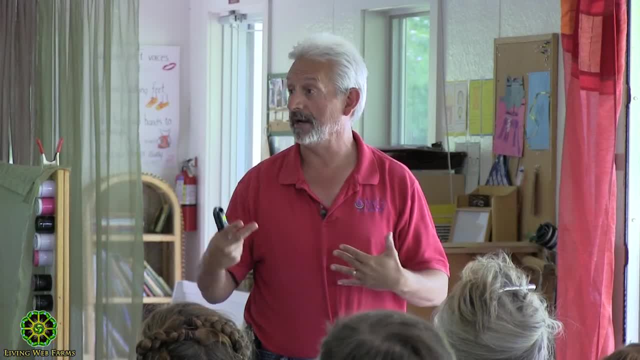 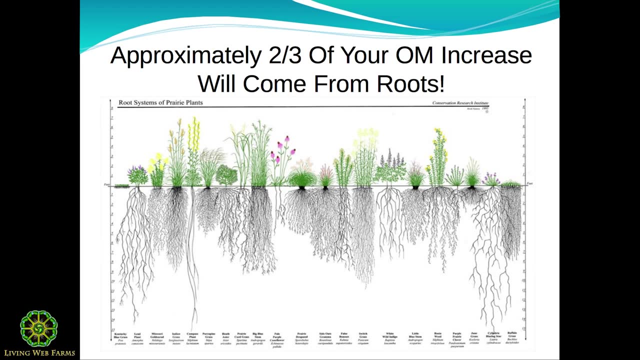 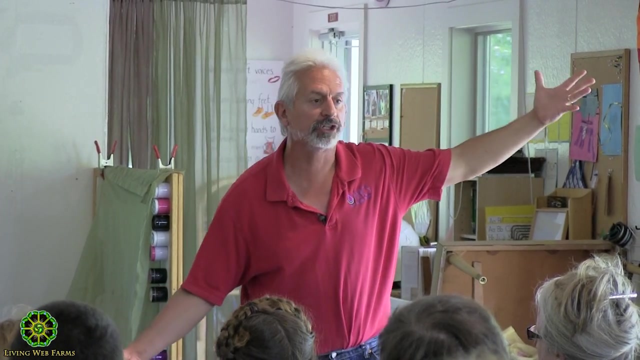 memory back. that's why you're gonna see a what. how many makes out there? do we have six, seven, eight mix? yeah, we're gonna mimic that architecture because they're captured nutrients differently, they all exude different chemicals. we're going to bring in 10. if you put a 10-way mix is like bringing a 10- 10 way rotation in. 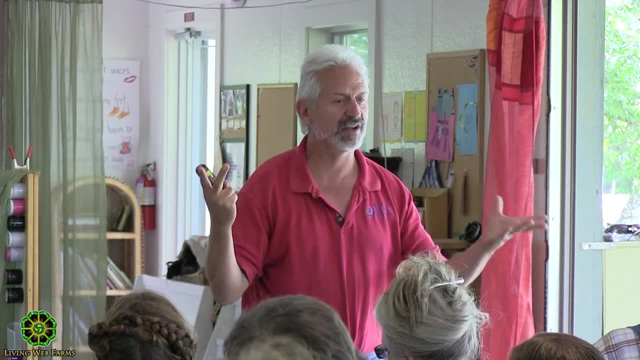 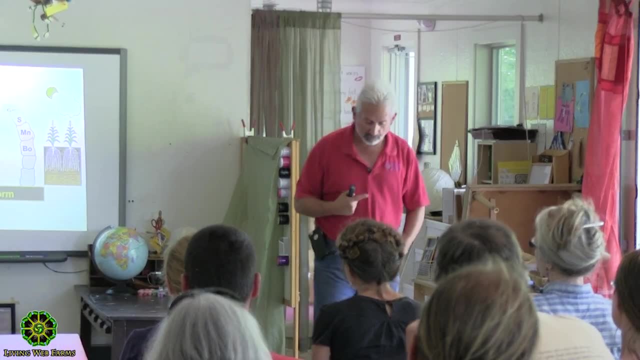 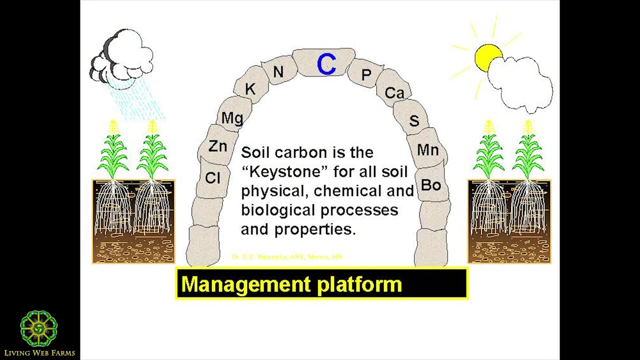 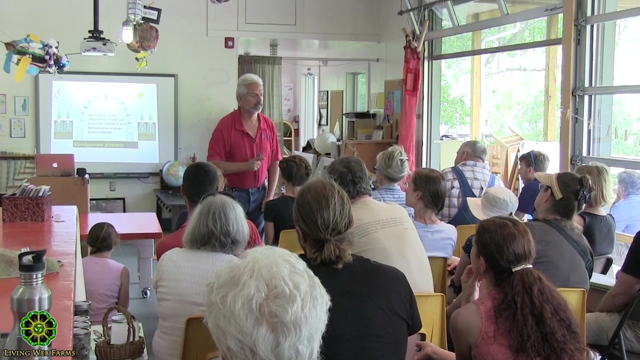 one year, we're capturing energy differently where and we're bringing ecological memory back. okay, this is the thing about. we need to realize this is the most critical nutrientос. nutrient in the soil, Carbon. Our soils are carbon depleted. Why is carbon the most critical? Because it's the bonding point of all the chemicals. It drives the system. It's the food that. 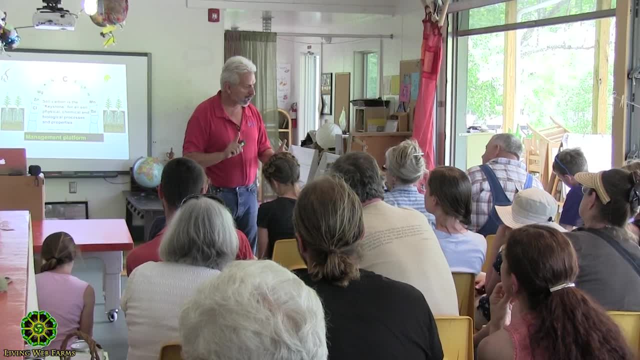 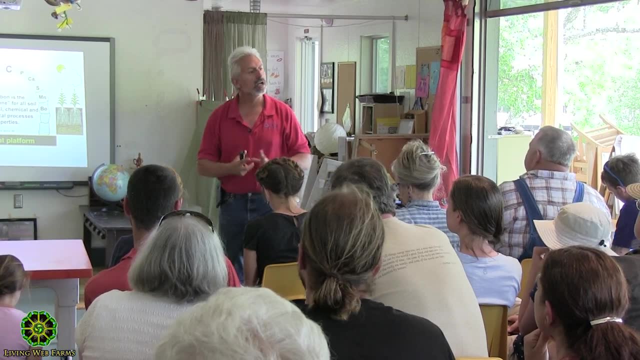 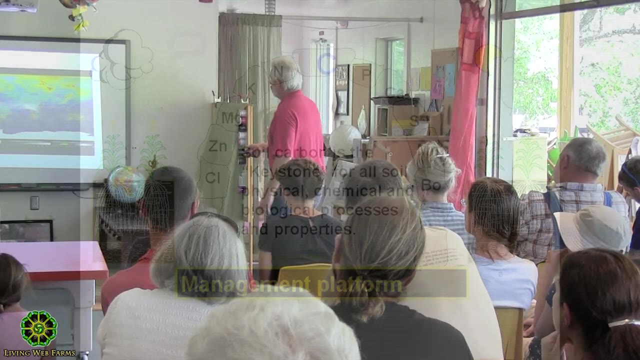 drives the biology. Our soils are so carbon depleted. this is why we have our issues. Carbon: They build the carbon, They run the system. It's carbon. Organic matter is 58% carbon. Okay, Now look what happened. I don't know if we have time for this. 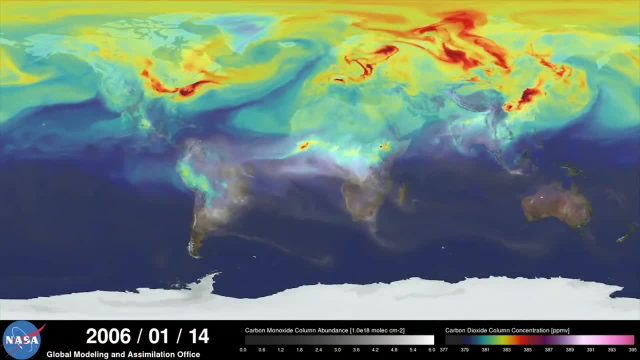 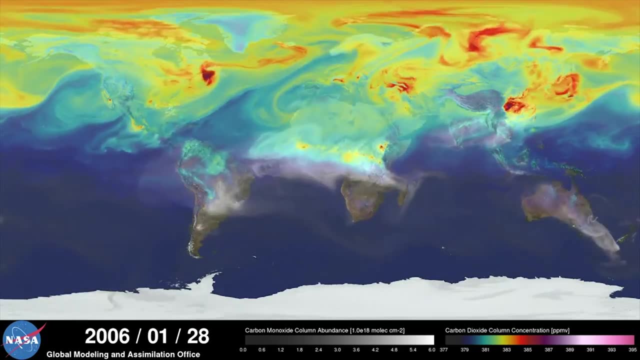 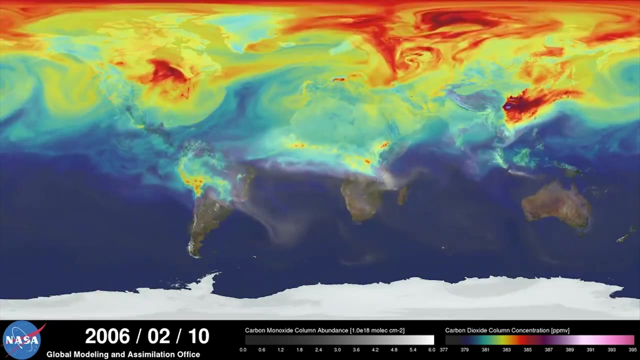 Well, let's just do this real quick because it's so cool. What you're looking at is a supercomputer model of carbon dioxide levels in the Earth's atmosphere. The visualization compresses one year of data into a few minutes. Carbon dioxide is the most important greenhouse gas affected by human activity. 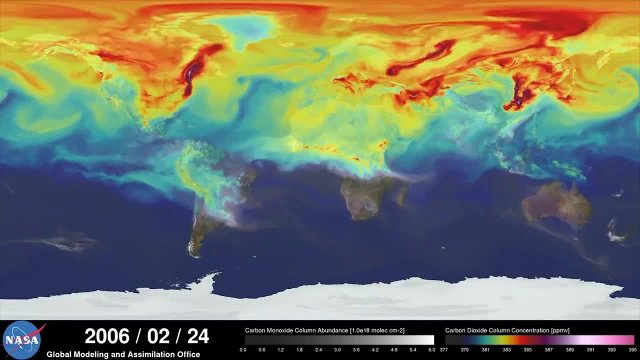 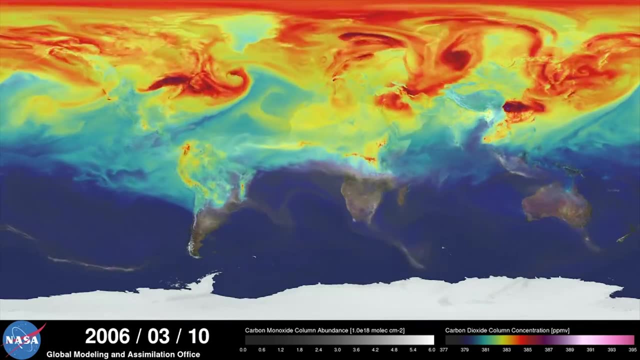 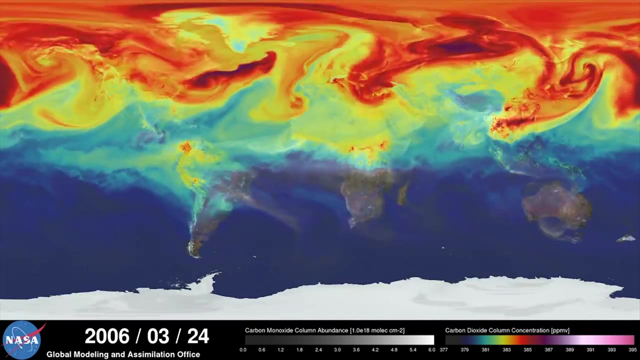 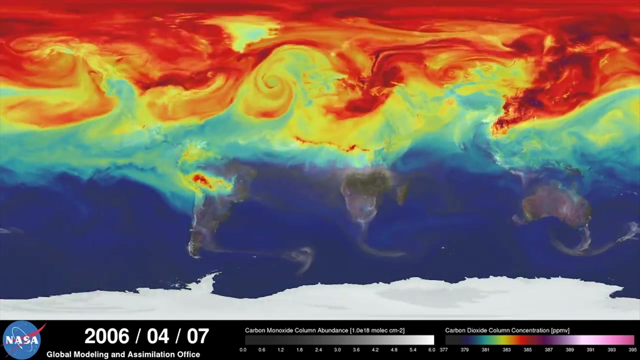 About half of the carbon dioxide emitted from fossil fuel combustion remains in the atmosphere, while the other half is absorbed by natural land and ocean reservoirs. In the Northern Hemisphere, we see the highest concentrations are focused around major emission sources over North America, Europe and Asia. Look at the date. Notice how the gas doesn't stay in one place. 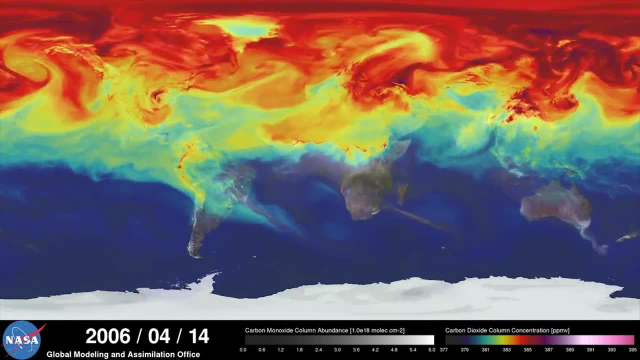 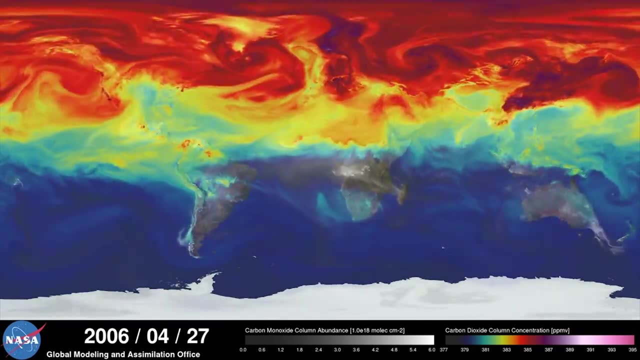 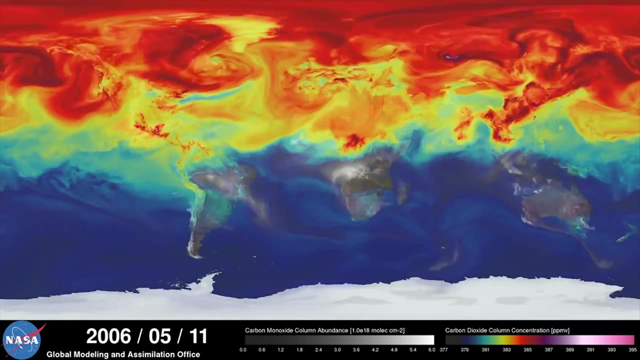 The dispersion of carbon dioxide is controlled by the large-scale weather patterns within the global circulation. What do we do in April? all over the country? See how it got red. We till Tillage is going on in that massive landscape area. During spring and summer in the northern hemisphere, plants absorb a substantial amount of carbon dioxide. 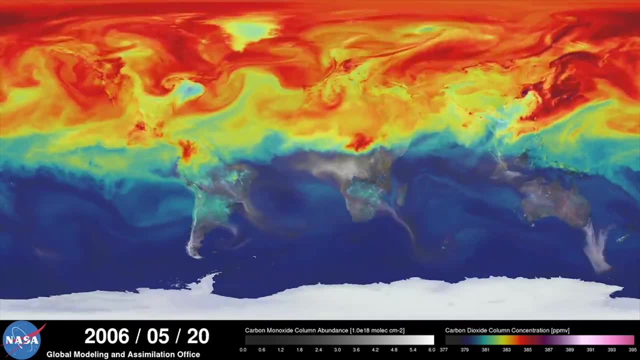 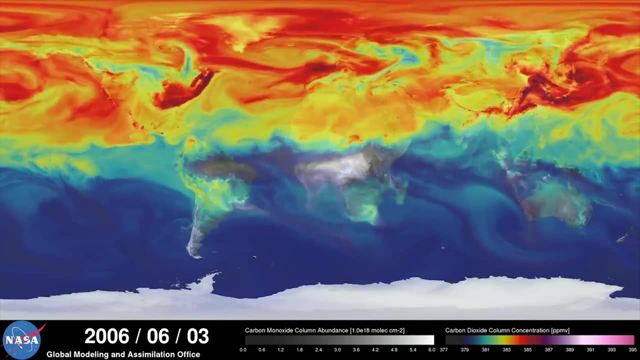 Now look when the plants start growing, Thus removing some of the gas from the atmosphere. Look at that. Look at me. We see this change in the model as the red and purple colors start to fade. Look at this. Oh yeah, baby. look at that. 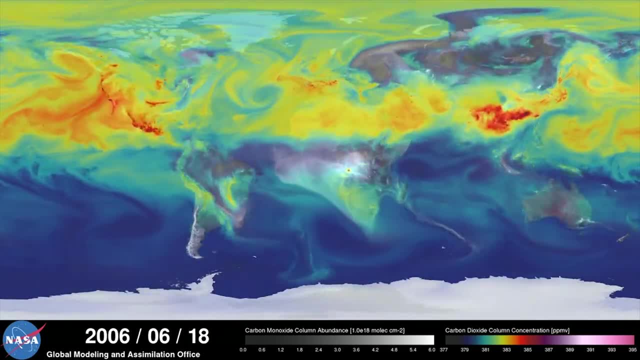 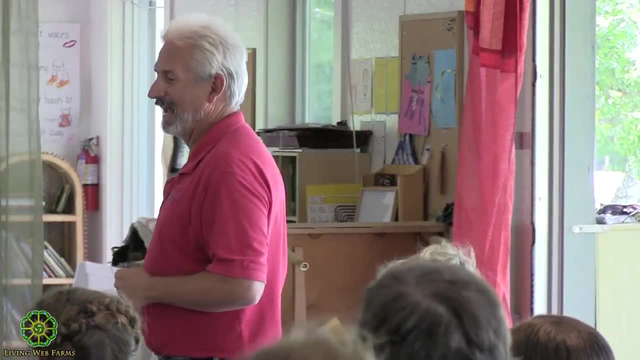 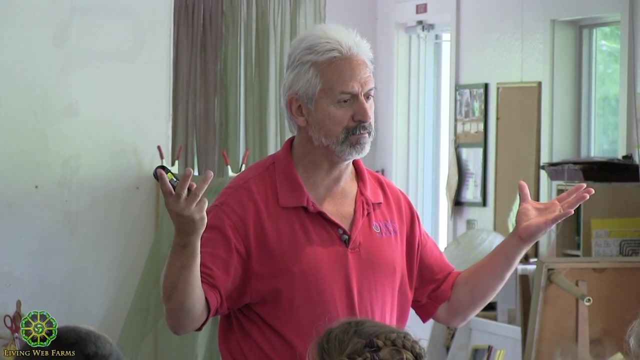 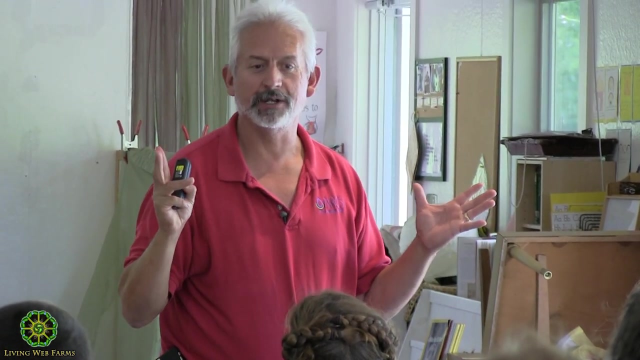 Do you mean if we covered the planet, we could fix our climate issues? Now, if we build our soils one to two percent organic matter, we could sequester all the CO2 that's been emitted by man in the last hundred years. If we build our soils one to two percent, 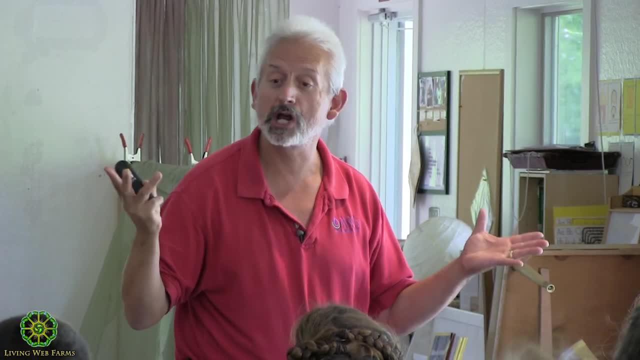 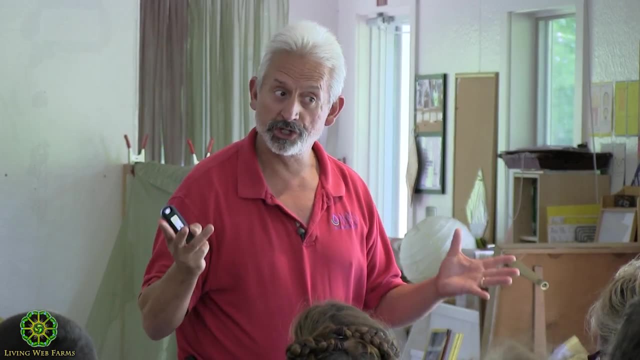 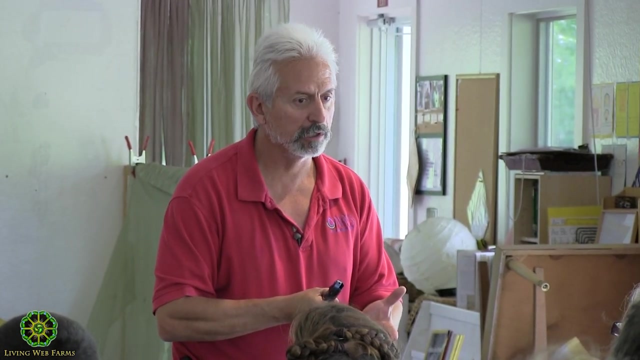 we could sequester all the carbon that's been emitted in the last hundred years. The second largest carbon sink in the world is the soil Ocean's number one, Soil's number two. You see how powerful this is. But most of our lands through the globe are uncovered. It was once all grassland.